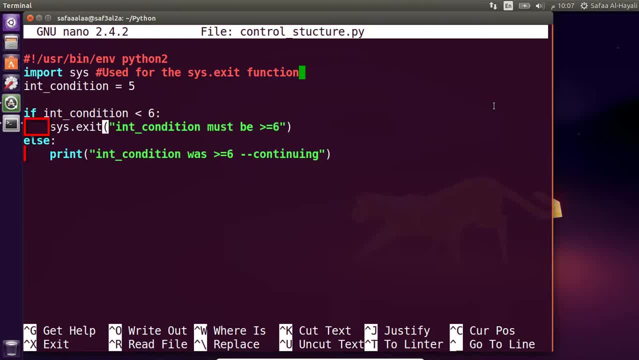 Notice that indentation, in this case 4 spaces per indent, is used to indicate which statement a block of code belongs to. Indentation is mandatory in Python, whereas in other languages sets of races are used to organize code blocks. For this reason, it is essential that you 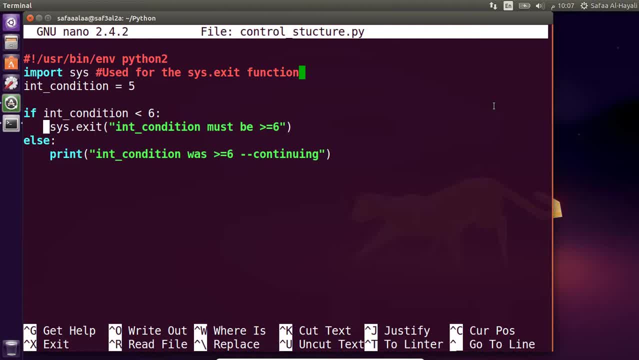 use a consistent indentation style. 4 spaces are typically used to present a single level of indentation. in Python, You can use tabs, but tabs are not well defined, especially if you happen to open a file in more than one editor. If statements are probably the 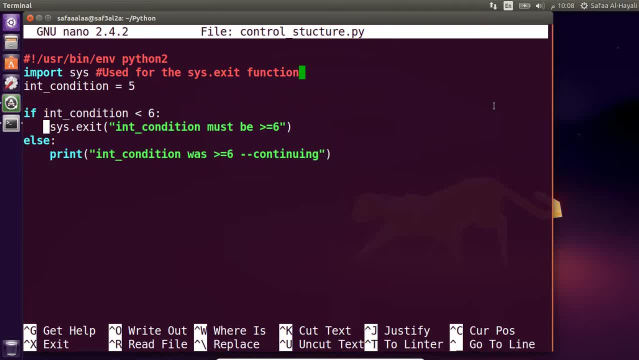 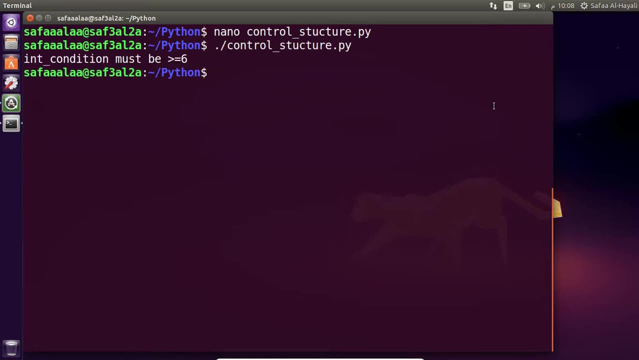 most commonly used control structures. Other control structures include force statements, which allow you to iterate over items in collections or to repeat a piece of code a certain number of times, While statements a loop that continues while the condition is true. We are going to write a program that will ask the user to input an arbitrary number. 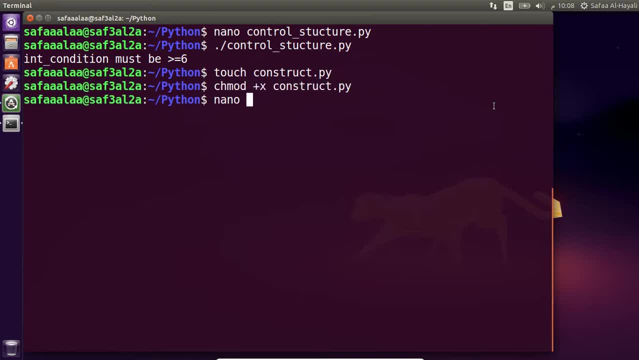 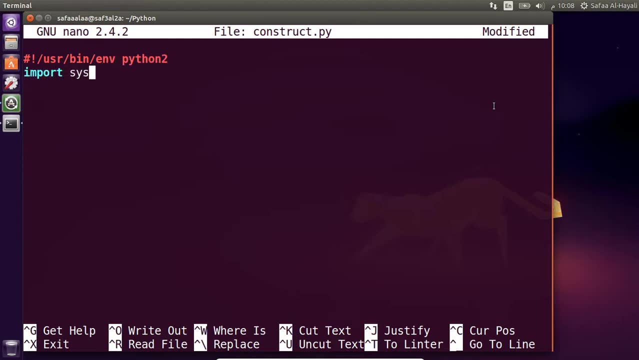 of integers, store them in a collection and then demonstrate how the collection would be used with various controls. Import system used for the systemexit function. I will define a variable to hold the number of integers we want in the list By now. the variable targetInteger contains a string representation. 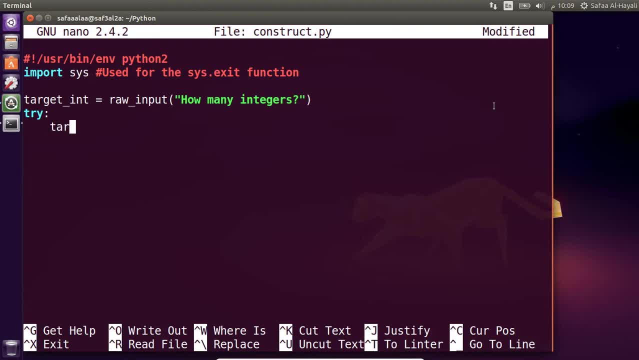 of whatever the user type. We need to try and convert that to an integer, But be ready to deal with the errors if it is not, otherwise the program will crash. We want to define a list to store the integers. Count variable is used to keep track of how many integers we currently have. Keep asking. 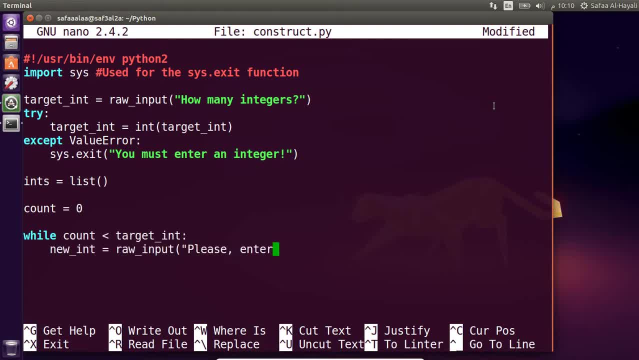 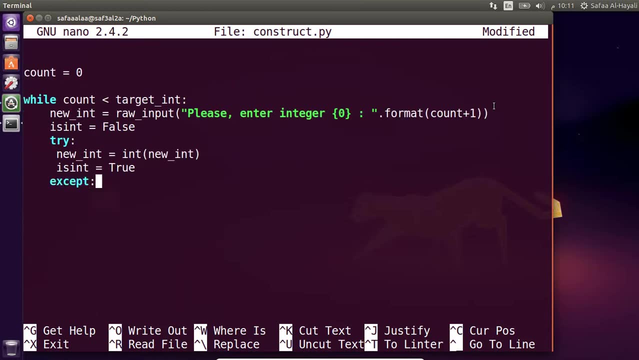 for an integer until we have the required number. If the evolve succeeds, then isInteger will be set to true. Only carry on until the integer is set to true. If the evolve succeeds, then isInteger will be set to true. Only carry on until the integer is set to true. 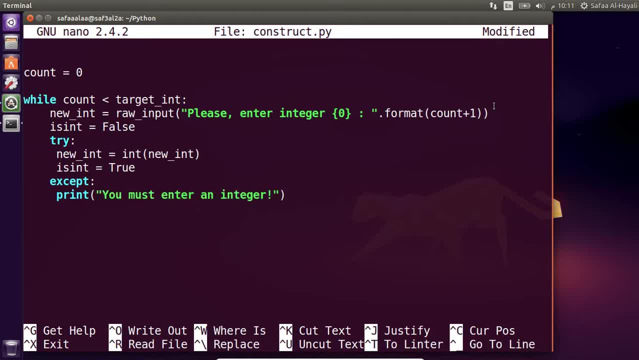 If the evolve succeeds, then isInteger will be set to true If we have an integer. If not, we'll loop again. Notice that I use double equals sign, which is different from the single equals. The single equals is an assignment operator, whereas the double equals is a comparison.